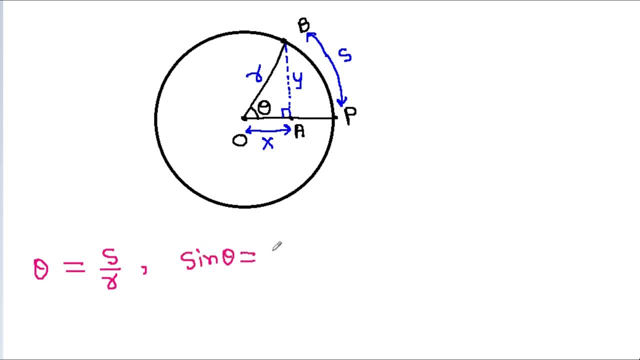 and sin theta will be equal to r And cos theta will be equal to x by r and tan theta will be equal to y by x. And now, if we have the same circle, and this is the center O, and this point is B, And if we decrease this point, then this point is A. 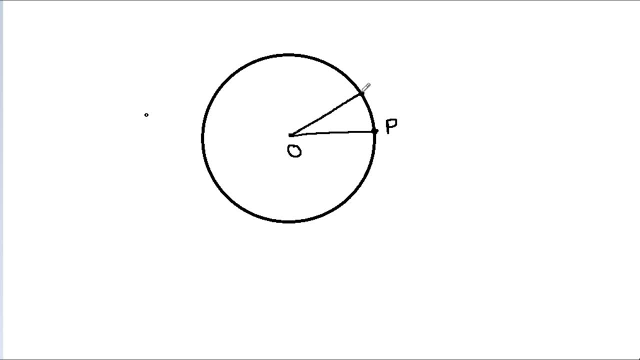 If we decrease the angle, suppose this is point B and this is theta, and theta is very small And this is the radius r, the arc length is s, And if we draw the power perpendicular from B, then this length will be x and this will be y. 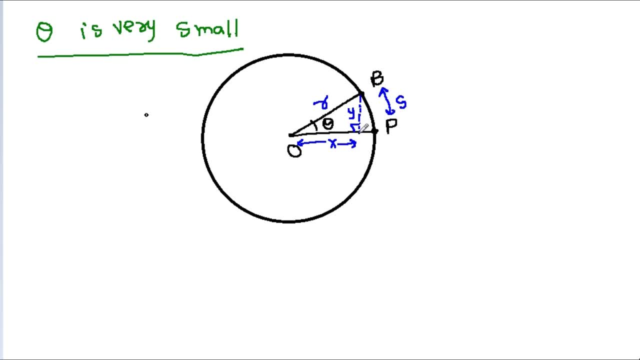 And this point is A. So from here we can say that if theta is very small, then y will be approximately equal to s and x will be approximately equal to radius r, And now we have: theta is equal to s. by r And sin, theta is equal to r. 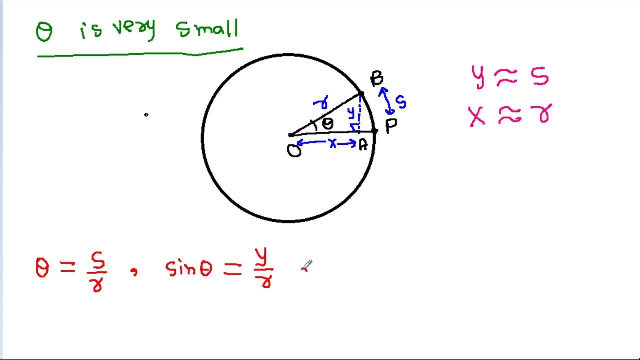 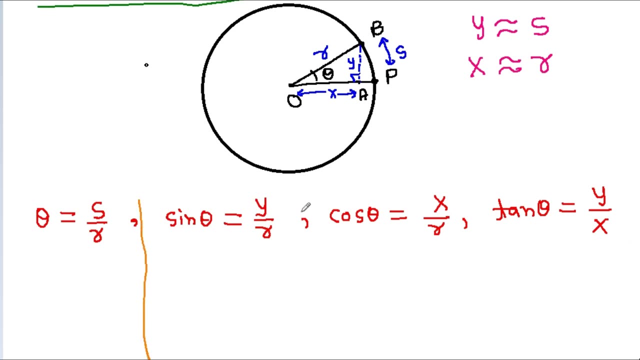 Sin theta is equal to y by r, Cos theta is equal to x by r, And tan theta is equal to y by x. And now sin theta is equal to: we have: y is equal to s, y is equal to s by r. 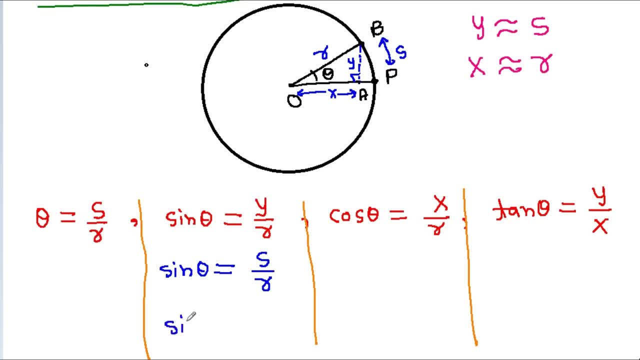 And s by r is equal to theta. So we get sin theta is equal to theta. And cos theta is equal to x is equal to r by r. So we get cos theta is equal to 1.. And tan theta is equal to y is equal to s. 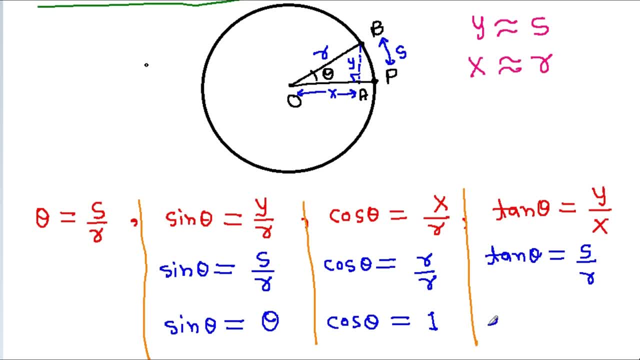 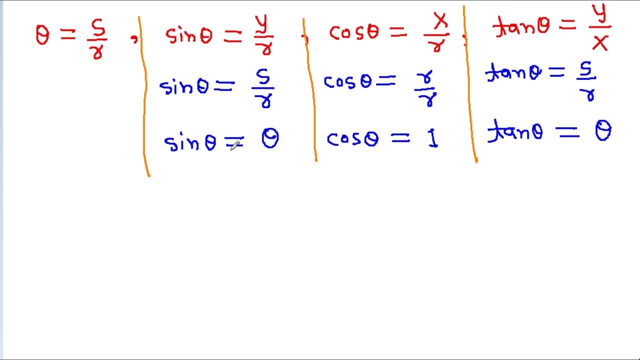 And x is equal to r And s by r is equal to theta, So tan theta is equal to theta. So for a small angle, sin theta is approximately equal to theta and cos theta is approximately equal to 1 and tan theta is approximately equal to theta. and note that theta is in radian. 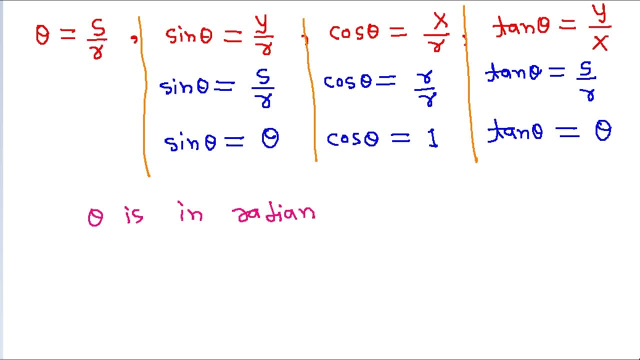 Because we have: theta is equal to s by r, that is in radian. So theta is in radian And now if we have to find the value of sin 2 degree, then we have to convert 2 degree in radian and we know that 180 degree is equal to pi radian. 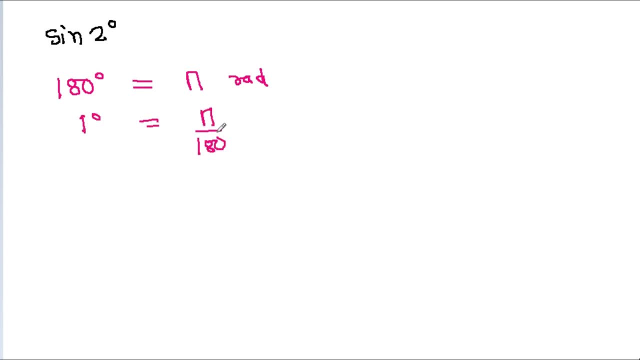 So 1 degree will be pi by 180 radian, And now sin 2 degree will be sin 2 into sin theta. Or we get sin pi by 90 radian. that is approximately equal to pi by 90. And if we have to find the value of tan 5 degree, then tan 5 degree will be equal to. 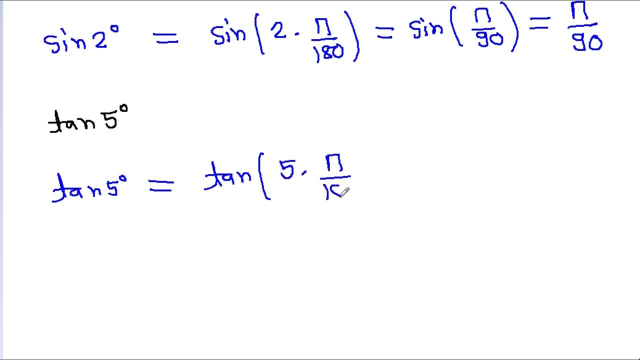 tan 5 into pi by 180 radian And it will be equal to tan pi by 36 radian. that will be equal to pi by 36. And if we have to find the value of cos 3 degree, then cos 3 degree will be equal to. 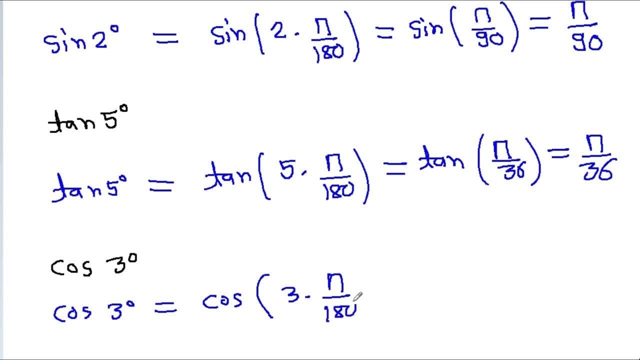 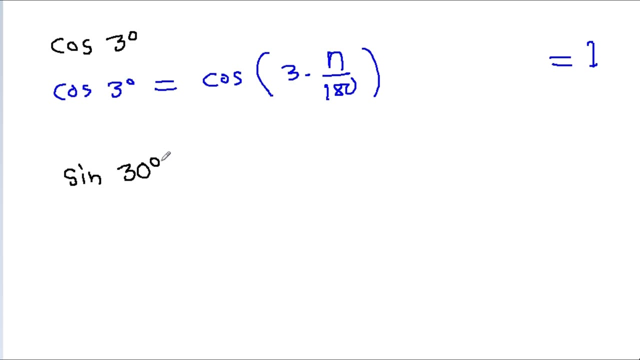 cos 3 into pi by 180 radian and cos theta. first one, theta, is approximately equal to 1.. And now If we have to find the value of sin 30 degree, then we know that sin 30 degree will be equal. 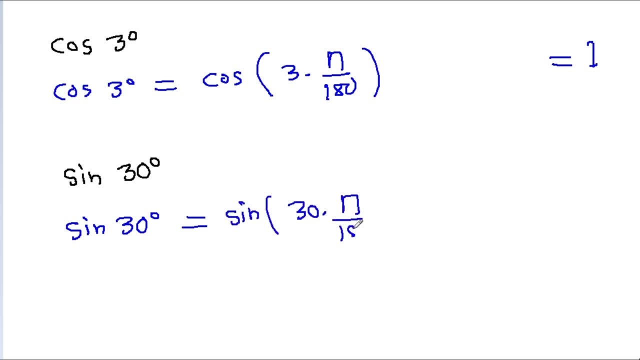 to sin 30 into pi by 180 radian, that will be sin pi by 6.. Now can I say that sin pi by 6 is approximately equal to pi by 6? Is it true? So it is false, Because 30 degree is equal to pi by 6..